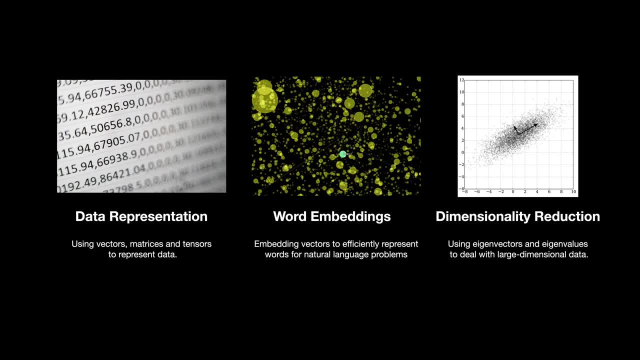 and dimensionality reduction. So data representation: you can basically represent your data using vectors, matrices and tensors And in word embeddings or vector embeddings, it is just about replacing a large dimensional vector with a smaller one. For instance, in NLP we deal. 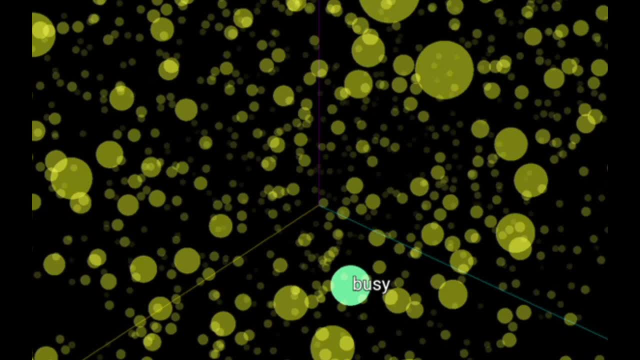 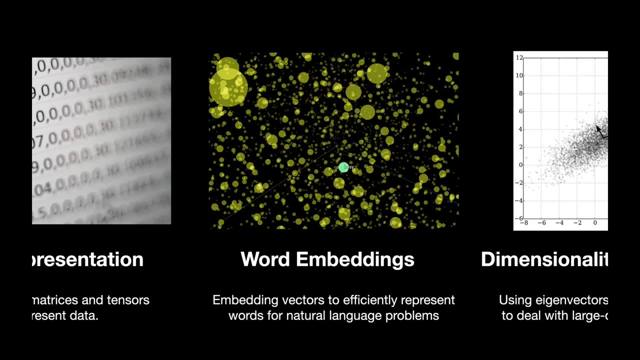 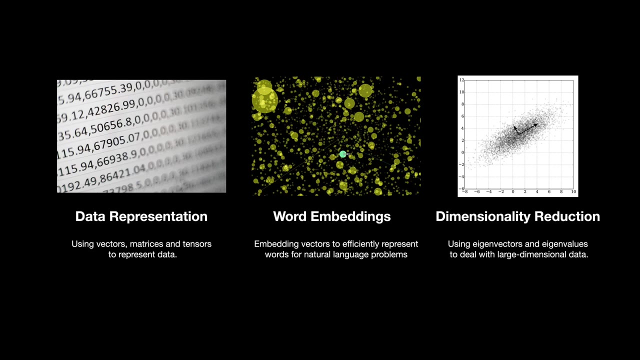 with a lot of textual data. We deal with so many words And each word represents a different meaning which might be similar to another word, but vector embeddings in linear algebra allow us to represent these words more efficiently. And finally, dimensionality reduction. So concepts like Eigenvectors allow us to reduce the 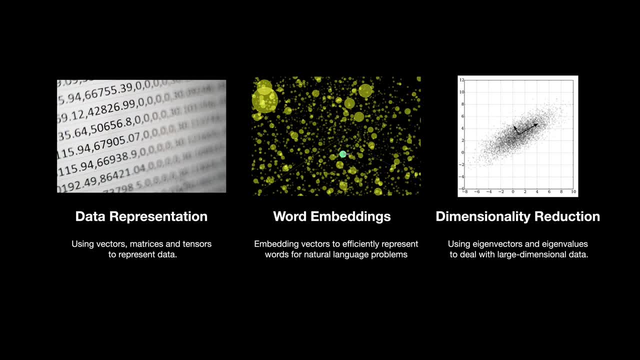 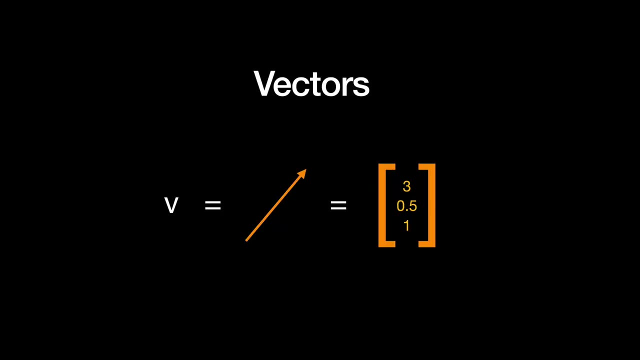 of features or dimensions of the data, while keeping the essence of all of them using something called principal component analysis, and all of it is actually driven by linear algebra, So we'll talk more about it in the course Now. linear algebra basically deals with vectors and operations. 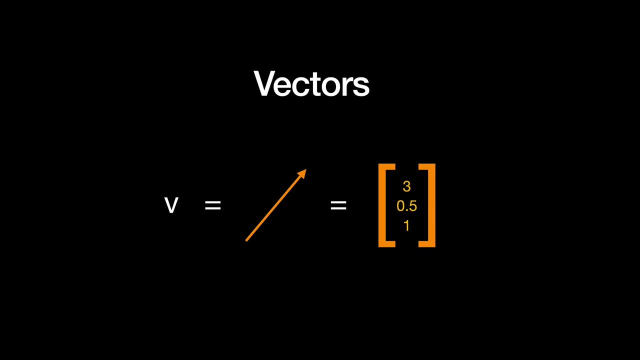 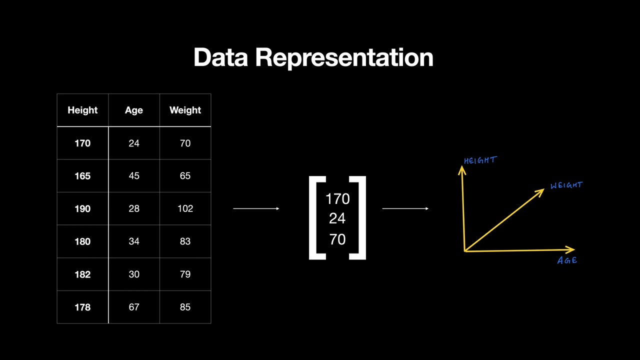 on vectors. So in NumPy this might be just a one-dimensional array of numbers, but geometrically this has both a magnitude and direction. So our data can be represented using a vector. For example, here, one row in this data is represented by this feature vector, which has three elements or 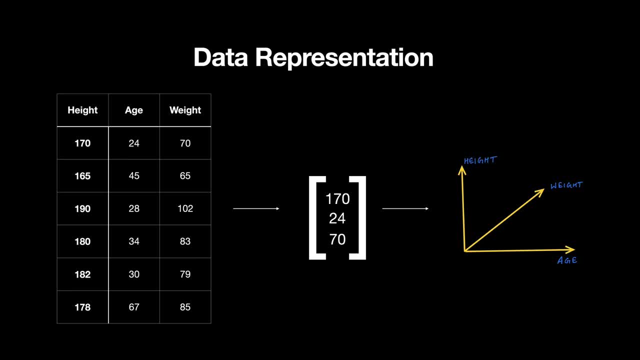 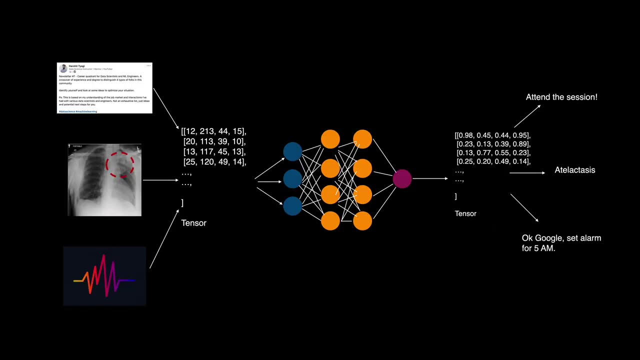 components representing three different dimensions. So n entries in a vector make it n-dimensional vector space and in this case we can see we have three dimensionals: height, weight and age. Now linear algebra can be seen in action across all the major applications today, be it sentiment analysis on a LinkedIn post or a Twitter post, be it detecting a type of lung. 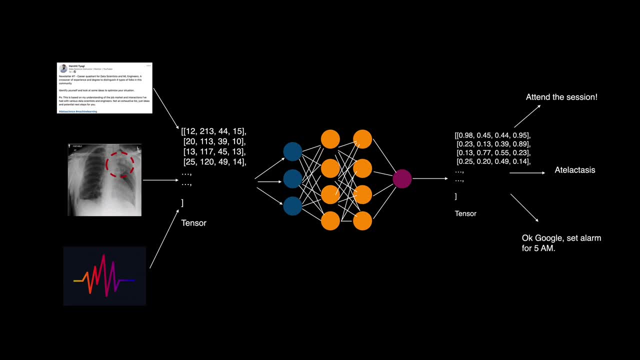 infection from an x-ray image or any speech to text bot. All of these data types are represented by numbers and tensors and we run vectorized operations to learn patterns from them using neural networks, which then outputs processed tensor again, which can be deduced to represent. 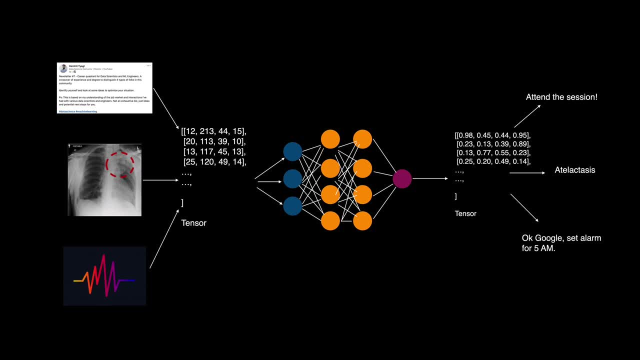 the final meaningful output. So here in the case you can see there's a lung infection x-ray image which is first converted into a tensor, then fed to a neural network. The neural network, after learning the patterns from these numbers, then outputs a learned tensor and then we finally 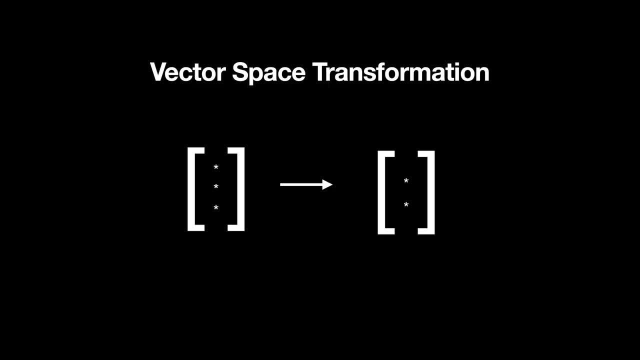 get the prediction from that output tensor. When it comes to embeddings, you can basically think of an n-dimensional vector being replaced with another vector that belongs to a lower dimensional space, which is more meaningful and the one that overcomes computational complexities. For example, here is a three-dimensional vector which is replaced by a two-dimensional vector. 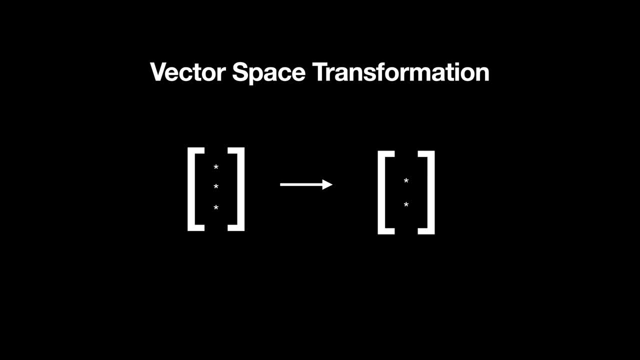 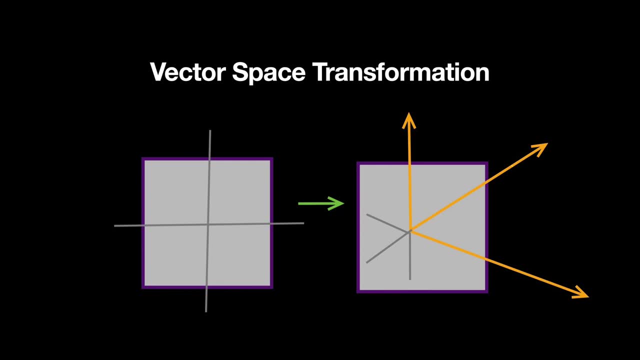 So you can basically think of a very large numbered dimensional space which is then converted into a lower dimensional space in a real-world scenario. Finally, you can think of embedding as a 2D plane being embedded into a 3D space, and that's where this term embedding comes. 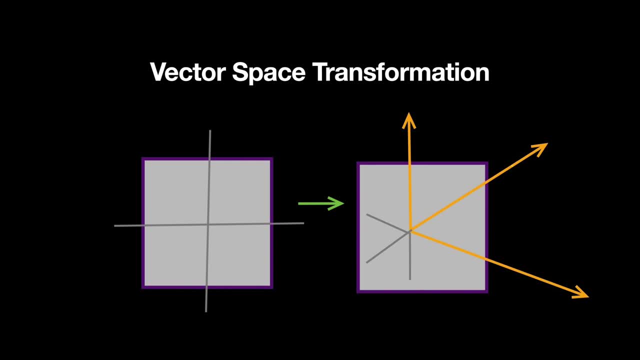 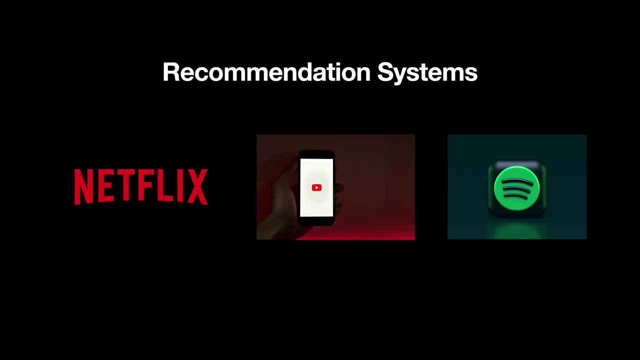 from You can think of the ground you are standing on as a 2D plane which is then embedded into the space in which we live. So that's the 3D space Now, just to give you a real world use case, to relate all of this discussion on vector embeddings, all applications that are giving you personalized 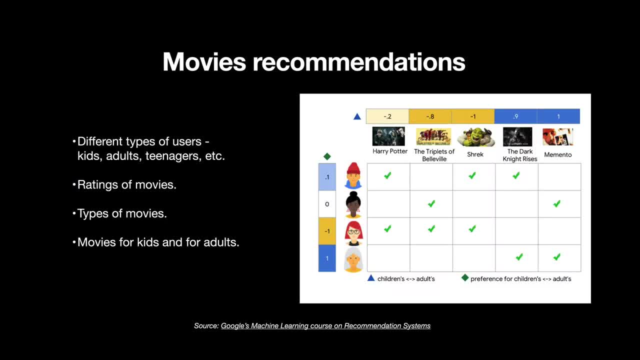 vector embedding in some form. For example, here is a graphic from Google's course on recommendation system, where we are given the data on different users and their preferred movies. Some users are kids and others are adults. Some movies were all-time classics, while others are more artistic. 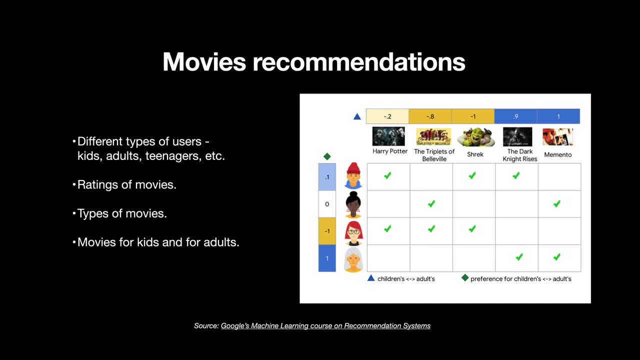 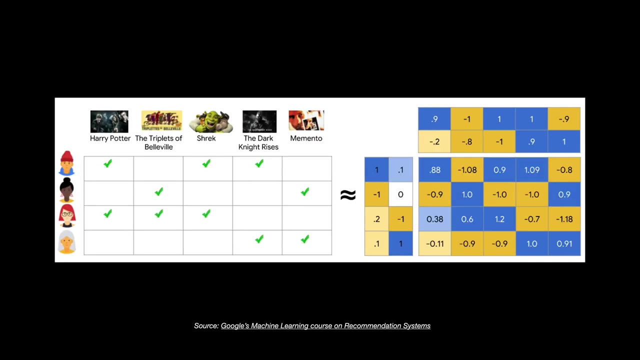 Some movies are targeted towards a younger audience- kids, while movies like Memento are preferred by adults. now we not only need to represent this information in numbers, but also need to find a smaller dimensional vector representation that capture all of these features. so a very quick way to understand how we can pull this task is by understanding something called matrix. 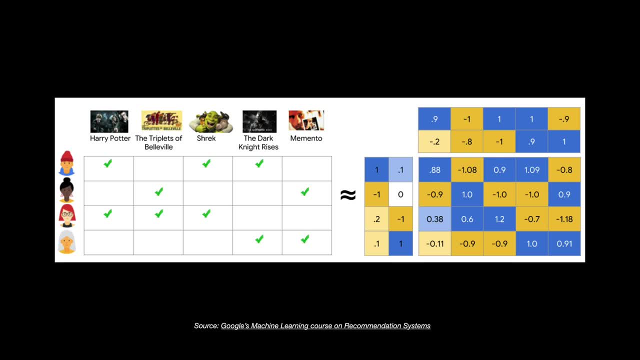 factorization, which allows us to break a large matrix down to smaller matrices. now ignore the numbers and the colors for now, and just try to understand how we have broken down one big matrix into two smaller ones. for example, here we have this matrix of four cross five, which is four. 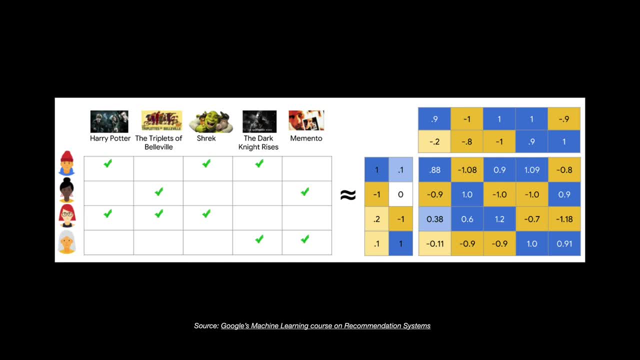 rows and five features, which was then broken down to two matrices, one of shape four cross two and the other of shape two cross five. we basically have new, smaller dimensional vectors for users and for movies- the whole one for the movies and the vertical one for the users- and this allows us to plot. 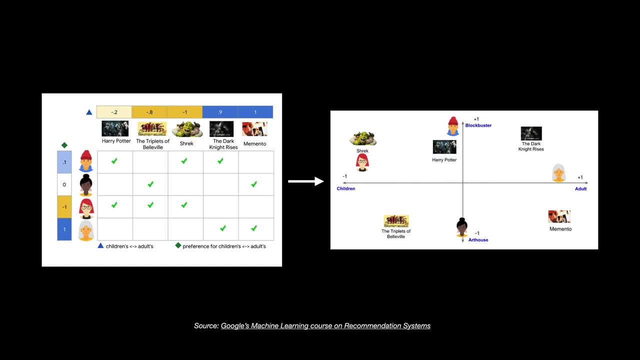 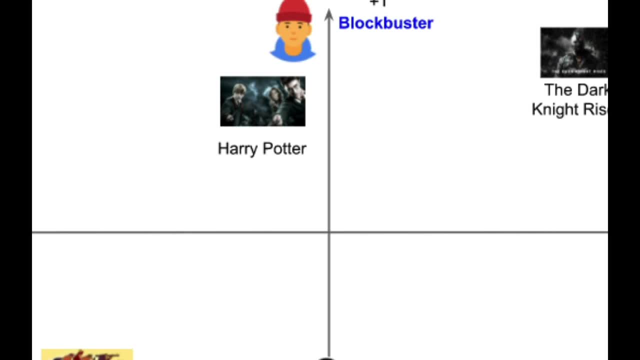 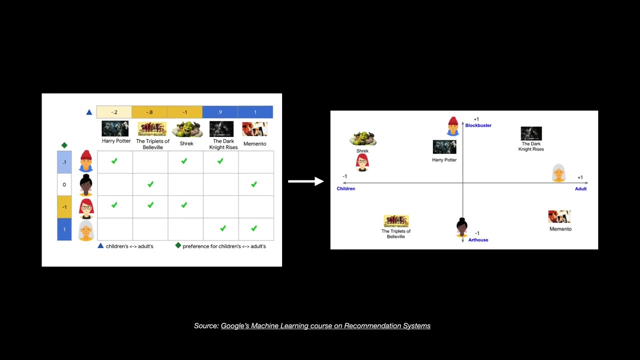 this on a 2d vector space, and here you will see that the user 1 and the movie Harry Potter are closer, whereas user 3 and the movie Shrek are closer. now you can basically relate that the movie Shrek is preferred more by kids, that's. 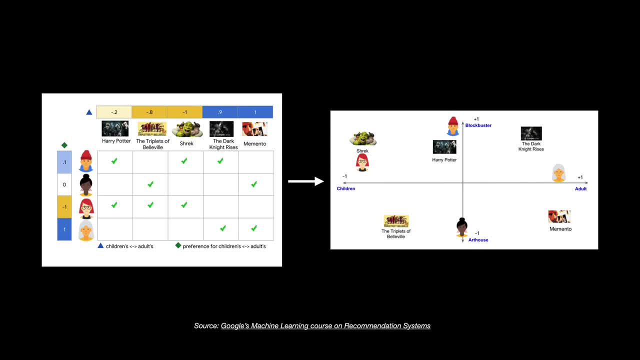 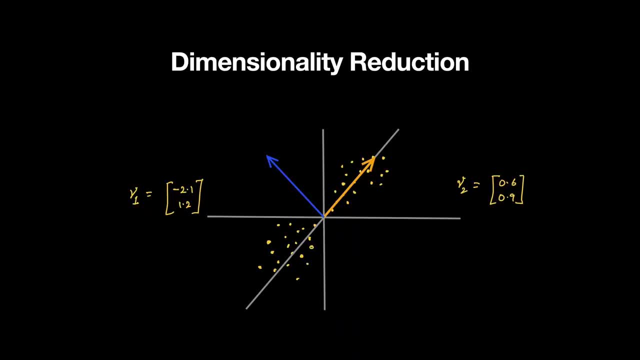 why they are closer. but the concept of dot product of vectors tell us more about the similarity of two vectors, which we will dive into in the course. with dimensionality reduction we have a goal: to narrow down our search and analysis to a lower number of dimensions and features. our data points are often. 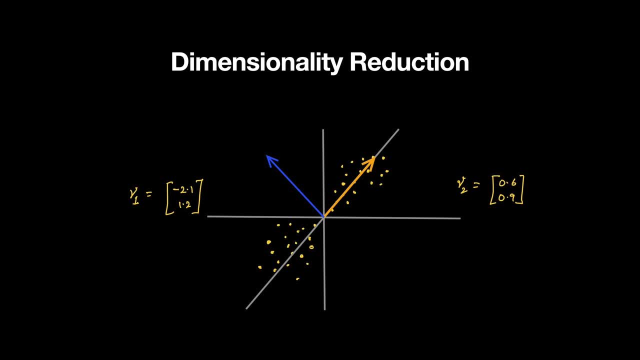 clustered along a line or a lower dimensional space, and we are basically looking for that principal direction that explains most of our data, and this is the principle that explains most of our data, and this is the principle that explains most of our data. and this is the done using the concept of eigenvectors in linear algebra, and the technique is called 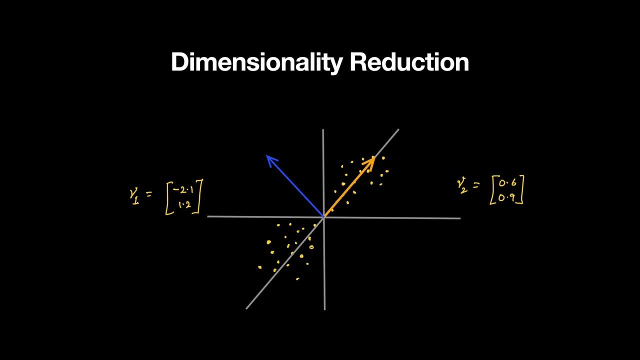 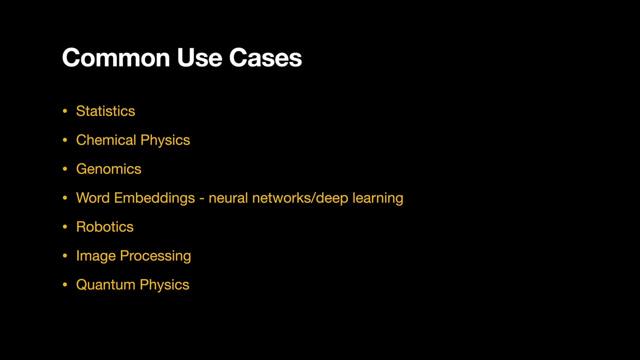 principal component analysis, which is widely used in unsupervised learning. Now linear algebra is driving a host of areas and to name a few, here is the list. It's basically used in statistics, chemical physics, genomics, word embeddings, neural. 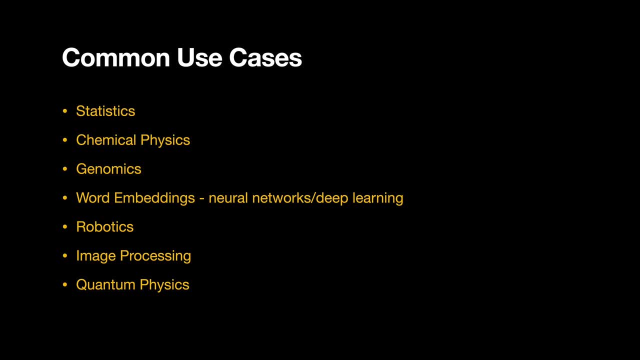 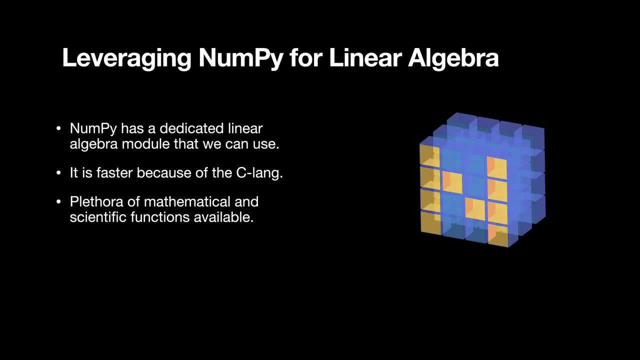 network, deep learning, robotics, image processing, quantum physics- you just name it. Now the question is: how is all of this possible in programming, and how can we learn to program these concepts of linear algebra? So the answer is: we don't have to reinvent the wheel. 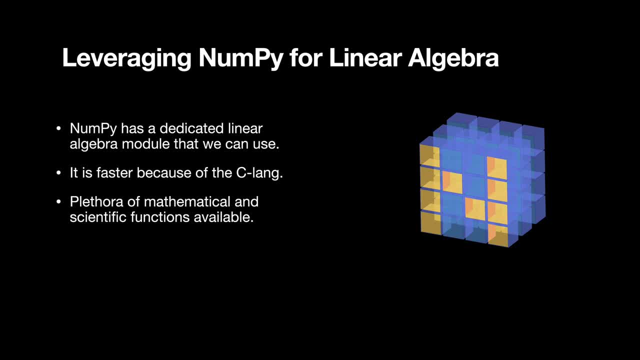 NumPy gives us access to all the underlying concepts of linear algebra. It's just about we need to understand the basics, the fundamental and the programming part of it. It's actually taken care of by NumPy. It is fast as it runs on compiled C code and it has a large number of mathematical and 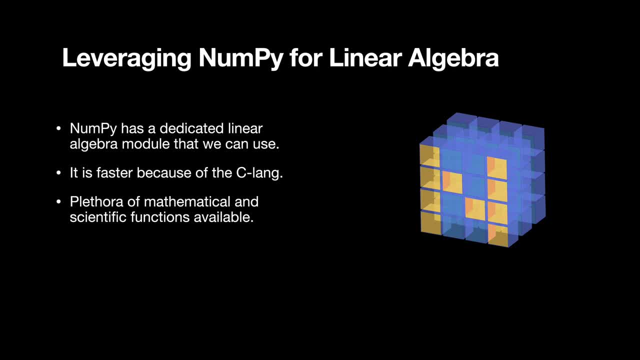 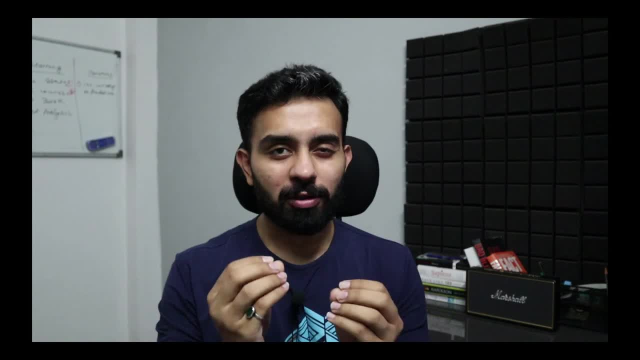 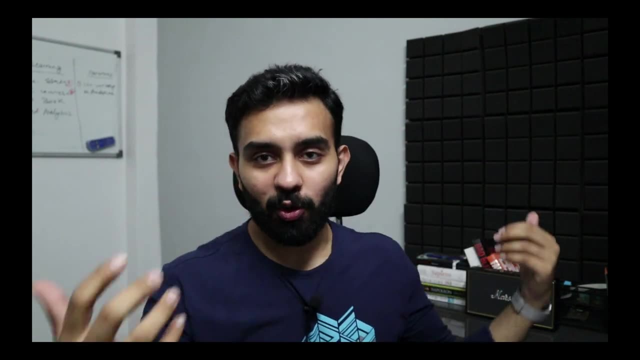 scientific functions that we can use. So I think that's enough context and motivation for learning linear algebra. Let's get down to it. So I hope you must have gotten some motivation, some understanding of how linear algebra is used in machine learning and you know everything that happens with model training or day to 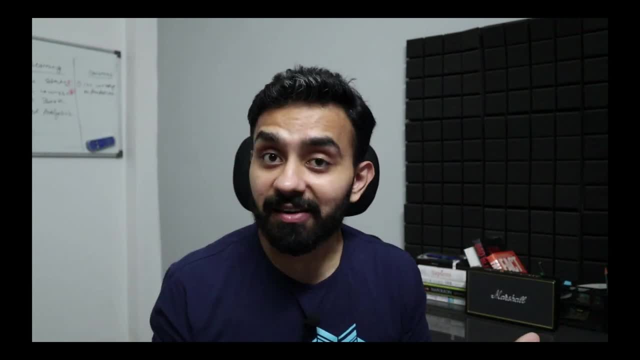 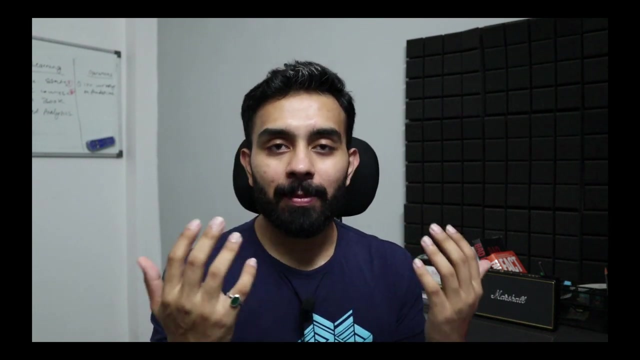 day representation or embeddings or, you know, dimensionality reduction for that matter. So you can find out different sort of resources on the internet. There are resources. I'm not saying my course is the only thing that's out there. But yeah, if you are comfortable with the mathematical notations, the deep learning, 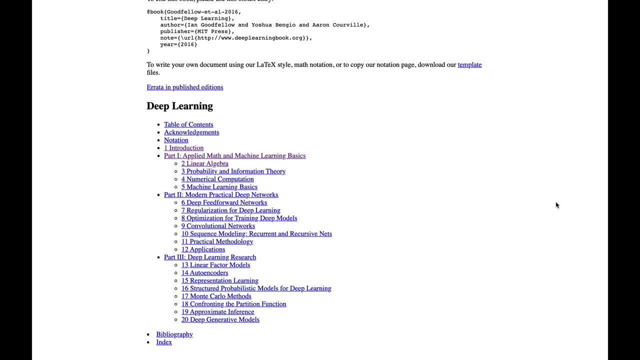 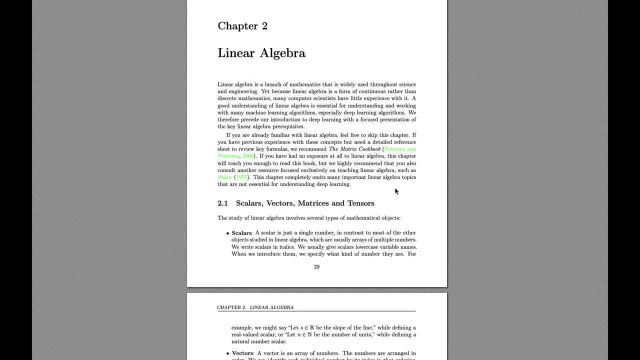 book by Ian Goodfellow and Yoshua Bengio. I think that's something that I would recommend. If you do not want to, you know, dive in too deep, Let's get down to it, And you don't want something that is very notational heavy, then you can definitely. 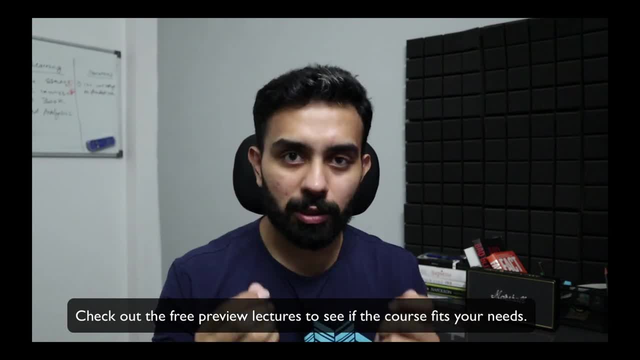 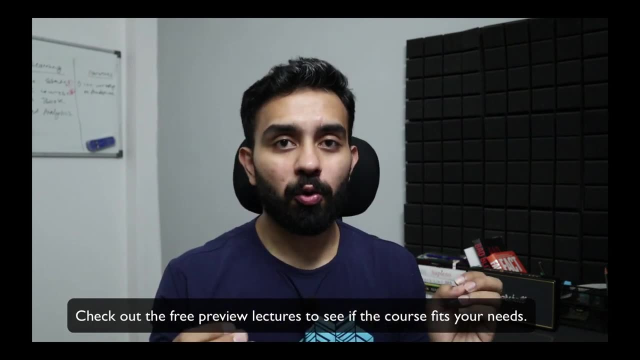 check out my course and I've covered it in very simple terms. So even if you think that you know you're not very good at mathematics, you can definitely easily follow that course. It's enough for you to get started with machine learning or data science. 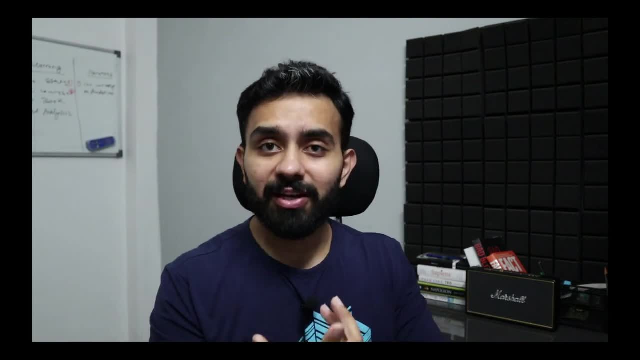 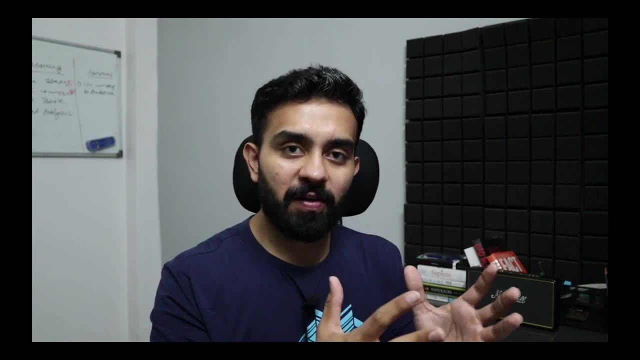 It covers statistics, It covers math, It covers calculus, linear algebra, the basic programming as well. So it's a whole package. If you want A specific part of it, Do let me know. You can always reach out to me at the email that's provided in the description. 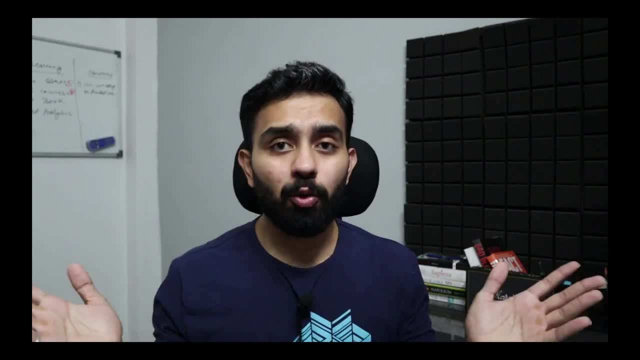 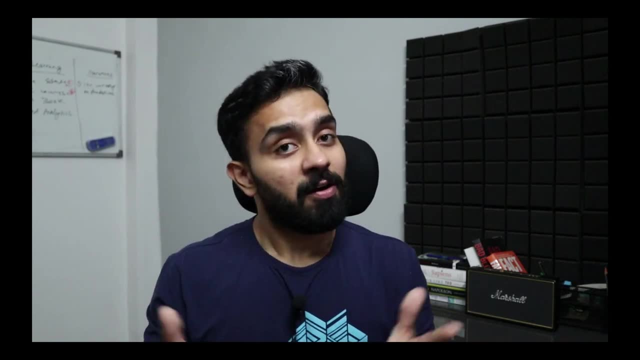 The course link is provided in the description as well. Feel free to ask any questions related to the course. I have provided the coupon code as well, which you can use to get $5 or 5.5 or, I think, 10% off on the launch price that I have set. 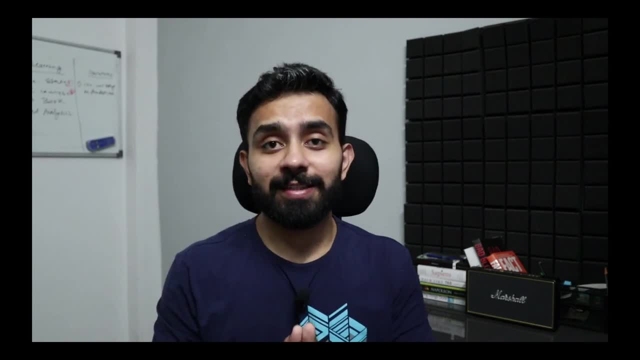 So, yeah, I am waiting for you to enroll and let me know in case you have any other queries. I can really help you out, sort out your questions and your queries. So until next time. this is Harsha Tyagi signing off. . . .